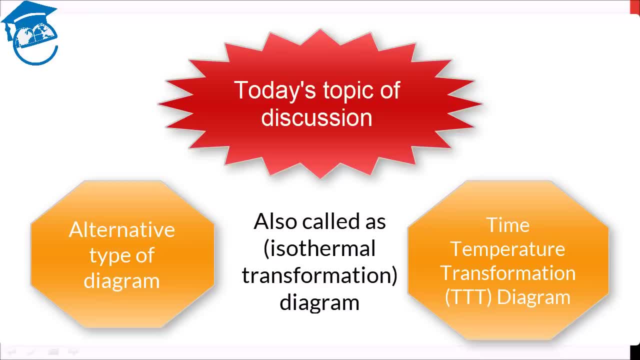 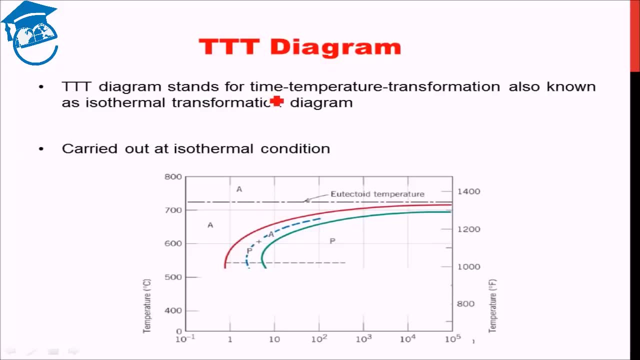 Transformation or alternatively, it is also called as Isothermal Transformation diagram. Let us see the terminologies involved. So basically, we are talking about transformation, but taking into account the time, ie the kinetics and the temperature involved. The alternative name says isothermal transformation diagram. 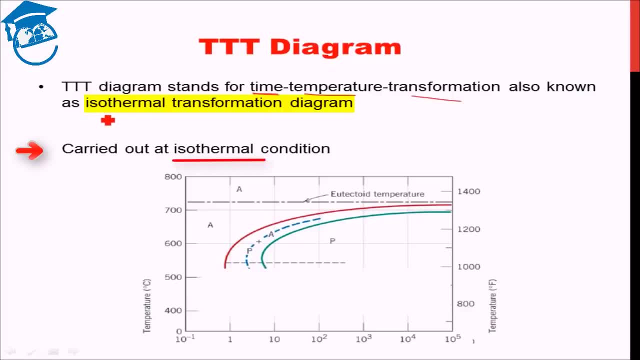 which means that this type of diagram deals with isothermal condition, ie the temperature present throughout the transformation, Isothermal transformation diagram. But if you come to think about it, isn't it similar to phase diagram, where you have equilibrium? Equilibrium means you are actually giving sufficient time for it to attain a particular temperature. 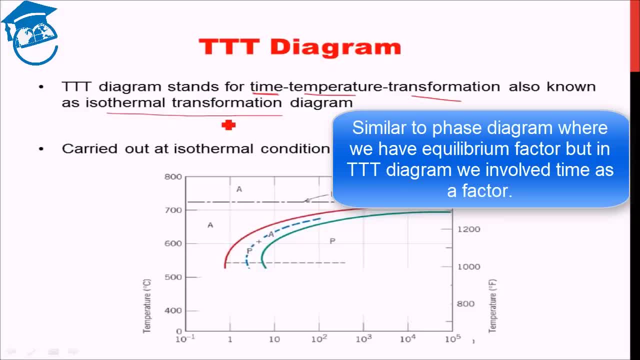 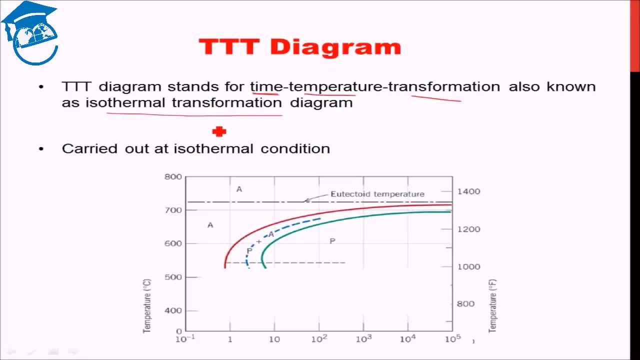 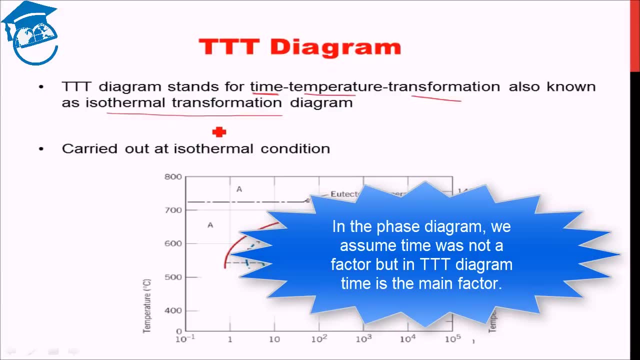 this is Sri 들어�ver diagram. So if we approach this diagram here, it is the TTT diagram. fundamental thing to understand is the amount of time that the materials maintained at one temperature In phase diagrams. we first assume that time was not a factor that at 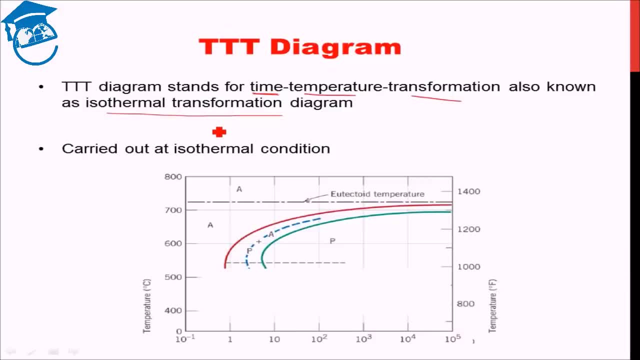 any moment equilibrium is established. Ok, so with the background, let us see what exactly is the TTT diagram. The TTT diagram looks something like this. This looks similar to the所以令我們 » проис abges 危� görün. 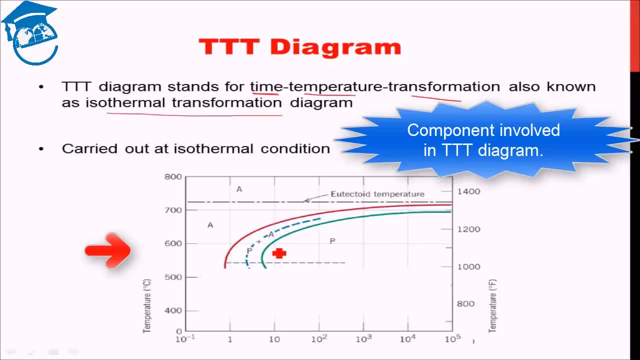 understand all the different components involved here. this axis, this axis is time, time, and it is plotted in logarithmic scale, because if we do not take log, then the effect cannot be observed, then the curve will be really, really elongated and as we saw in the previous relation, the previous lecture, 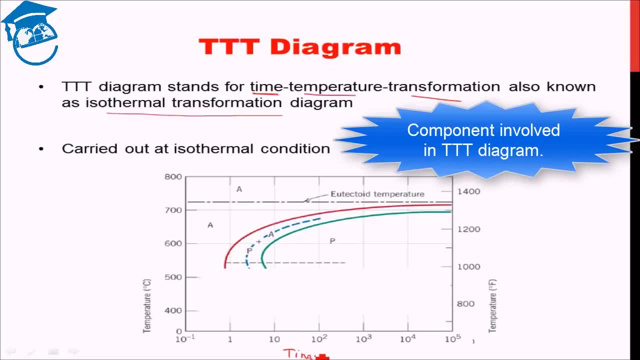 that the abrami relation is a exponential relation of time. therefore, we require a time component which is in logarithmic scale. this axis is our temperature axis. it can be in degree Celsius, it can be in degree Fahrenheit, doesn't matter. now let us consider the eutectoid composition itself, just to 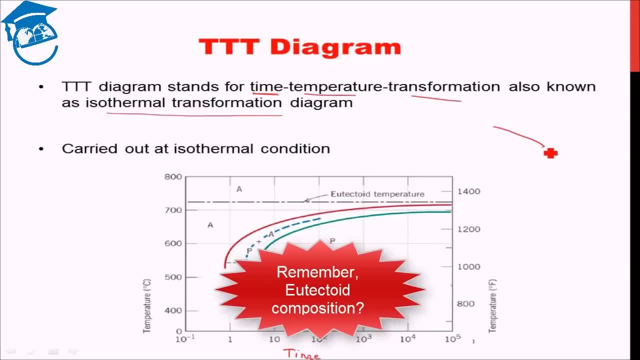 remind you what was the eutectoid composition. it was gamma here, transformation taking place, ferrite plus cementite at 727 degree Celsius, and this composition was 0.76 percent carbon. right, this was the eutectoid transformation and this was the phase diagram representation of it. 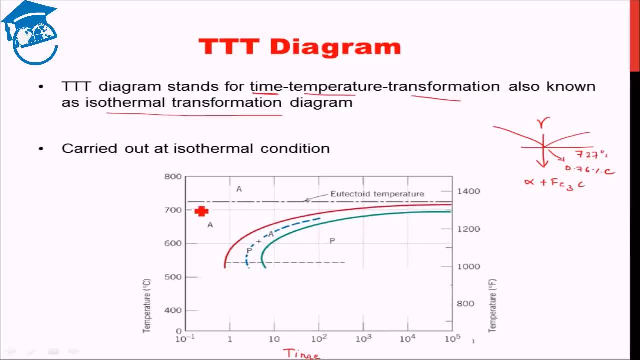 but in the TTT diagram what we do is that we draw the eutectoid temperature, which is 720 degrees Celsius, and then these curves shows the actual start and finish of perlite. this is the perlite start curve and this is perlite finish curve. what does this mean? 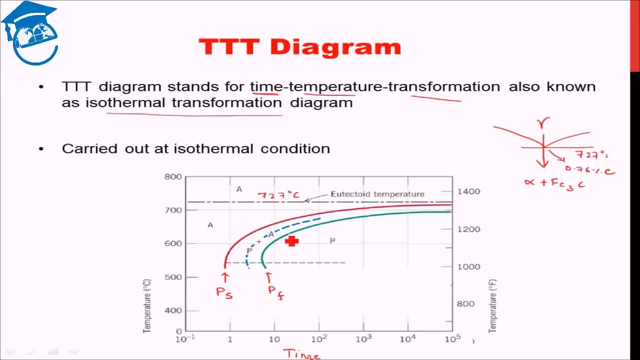 this means that ideally austenite should be present only till 720 degrees Celsius. right below that we should instantaneously have perlite if we go just via phase diagram. but in reality kinetic needs to be taken into account. so let's say that we start the time. we start from 800 degree Celsius, we cool it down to. 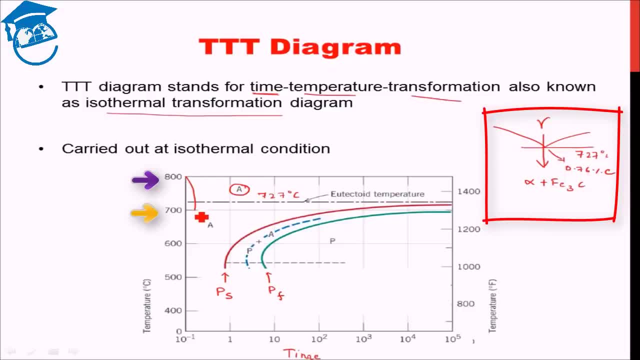 let's say 700 degree Celsius very quickly, and now we hold it at 700 degree Celsius. we hold it at 700 degree Celsius. now we add base natural ДиD and we hold it at 700 degree C celsius. we hold it at 700 degree Celsius. now we hold it at 700 degree C. 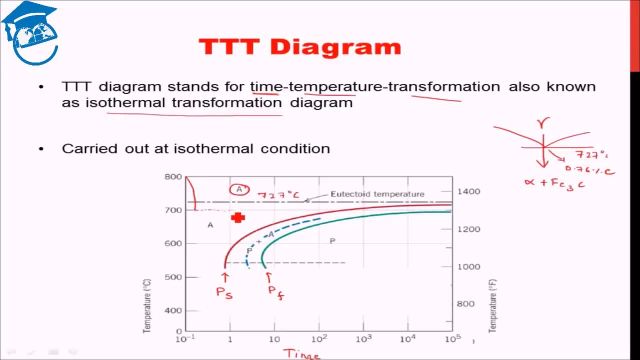 celsius. we hold it after 700 degree C celsius. if we will add the raw and artificial stress, then we change it to the clues a little bit more. per lth. we hold it at 1 second. still we have 100% austenite. we do not have any pearlite till. 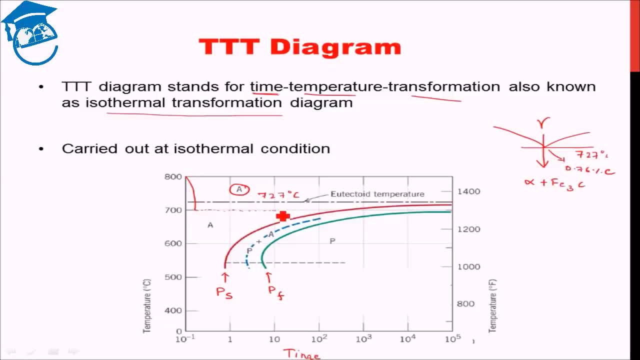 now we keep it at 700 degree celsius, at 10 second also, pearlite hasn't started to form. at 100 second, pearlite hasn't started to form. finally, over here, which is somewhere might be around 500 seconds, pearlite starts to form. this is pearlite start curve till this moment. 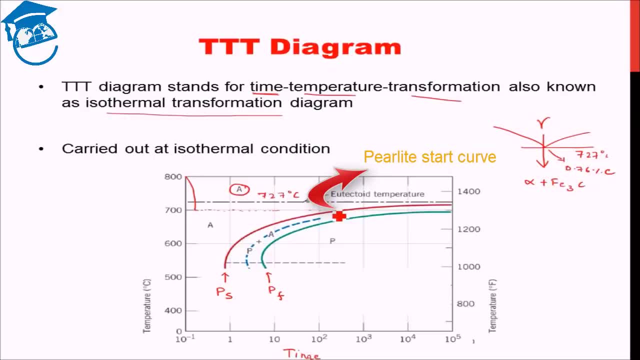 everything which we have was 100% austenite. we did not have pearlite here. pearlite starts to form. ok, beyond that, let's say we are over here at 1000, almost 5000 seconds. we have attained only about 15 seconds. 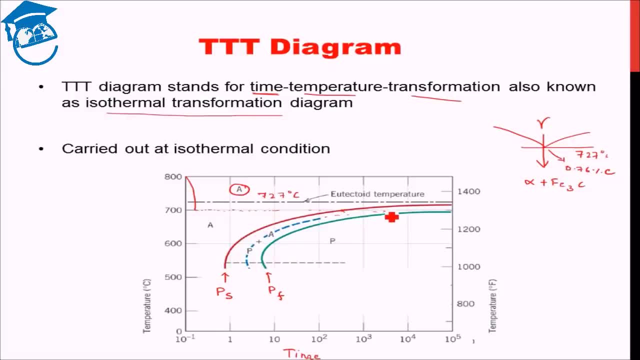 So we have attained only about 15 seconds. So even at this location we are 50% pearlite and 50% austenite. in order to get 100% pearlite at 700 degree celsius, we need to maintain the temperature for really really long time. 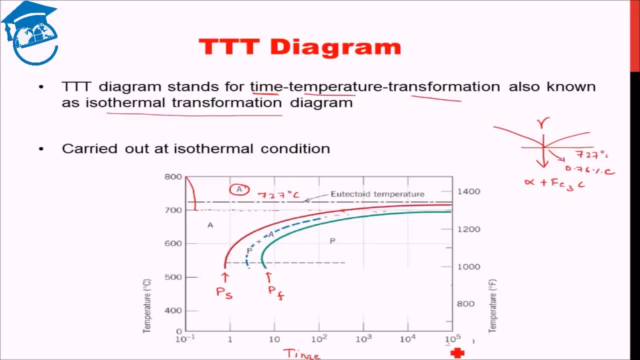 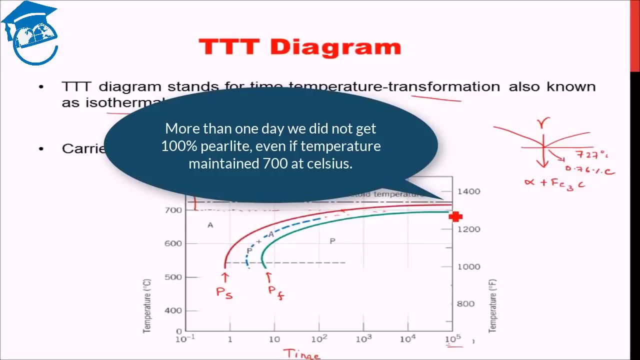 as you can see, even at 10 to the power 5 seconds, it is not cutting the 700 degree celsius isothermal line, is not cutting the finish curve. pearlite finish curve, that means even at 10 to the power 5 seconds, that is more than one day. we do not get 100% pearlite if 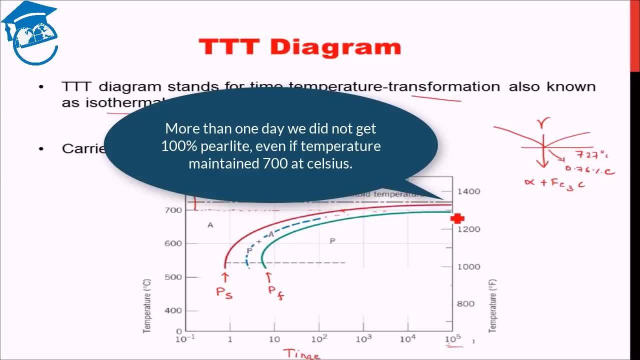 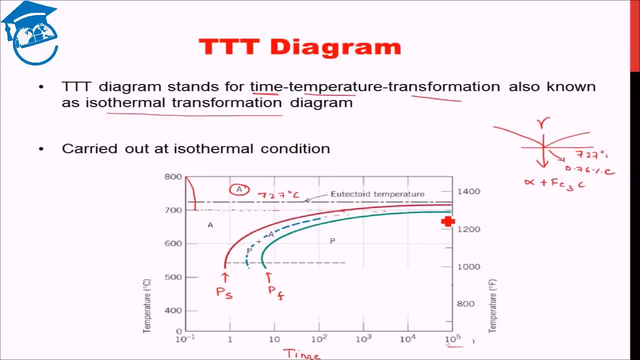 we maintain 700 degree celsius. ok, so you see how different is it from the thing which we saw in the phase diagram. phase diagram just assumed equilibrium and instantaneously you had pearlite, but here, at 700 degree celsius, which is actually under cooling of 27 degree. 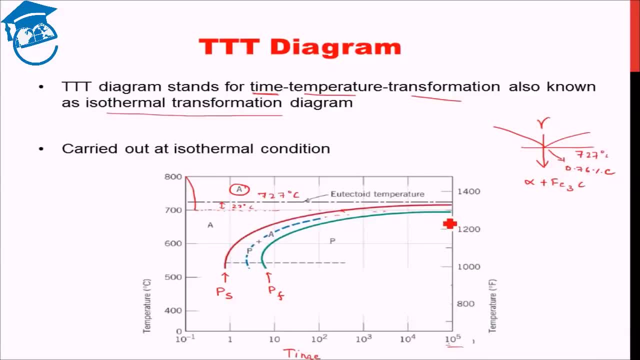 celsius, you do not get 100% pearlite, even after one complete day. now, alternatively, let's think that we take it down to 600 degree celsius. then pearlite starts forming at about 2 seconds and pearlite is completely formed. 100% pearlite is formed before 10 seconds. ok, see the interesting. 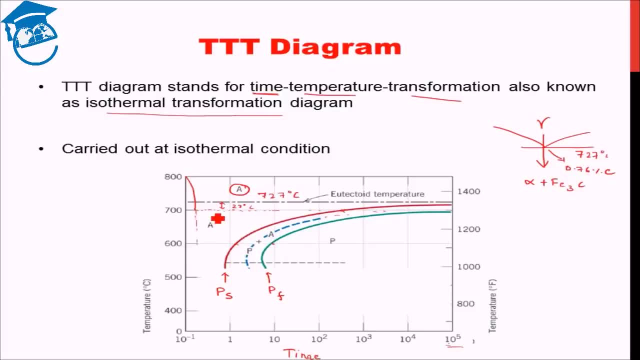 thing here. Ok, At 700 degree celsius, one day was not sufficient for 100% pearlite formation. at 600 degree celsius, under 10 seconds we get 100% pearlite. so that is the power of TTT. diagram it in a very concise. 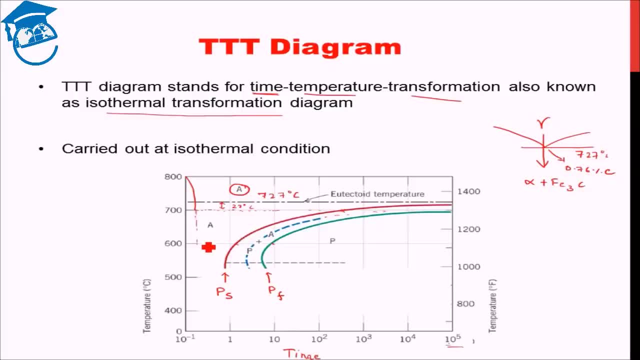 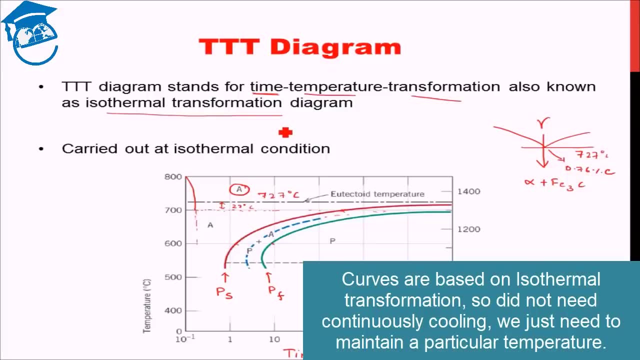 diagram packs a lot of information, a lot of heat treatment information. ok, and TTT diagrams are drawn in such a way that these lines, These lines are the lines, These lines are the lines are actually based on isothermal transformation condition, so you cannot continuously keep cooling. 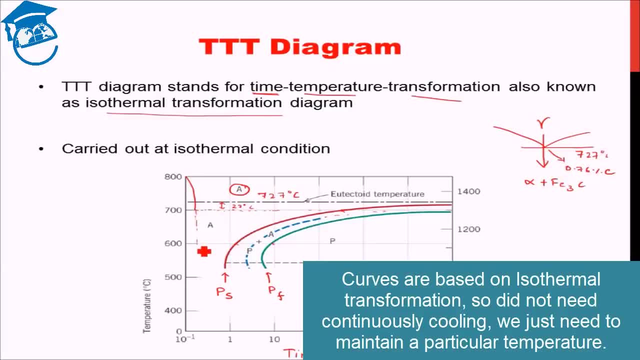 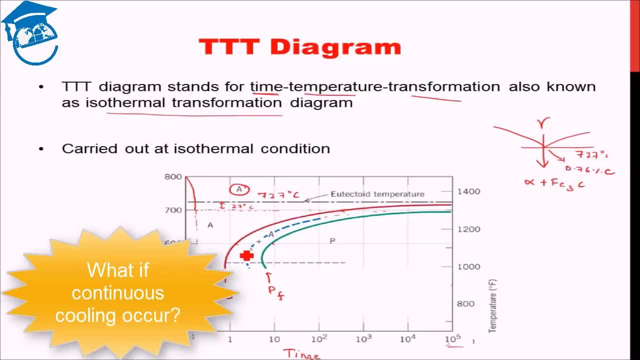 you need to hit a particular temperature and maintain that temperature. that's why isothermal. but in reality that won't be always the case. there will be cases where there will be continuous cooling. for that we'll discuss in our next lecture something known as cct diagrams- continuous cooling. 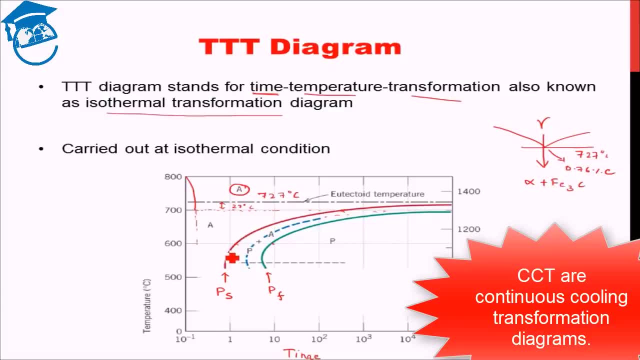 transformation diagram. but for now we assume that we are in the heat treatment categories where the temperature is maintained isothermally okay. so just to recap, this was pearlite start, this was pearlite finish. anywhere in between you have certain amount of pearlite formed and remaining. 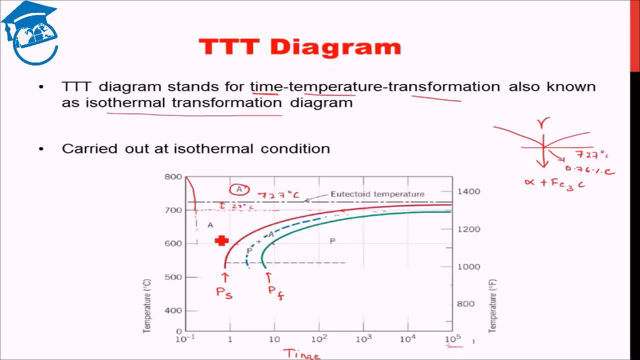 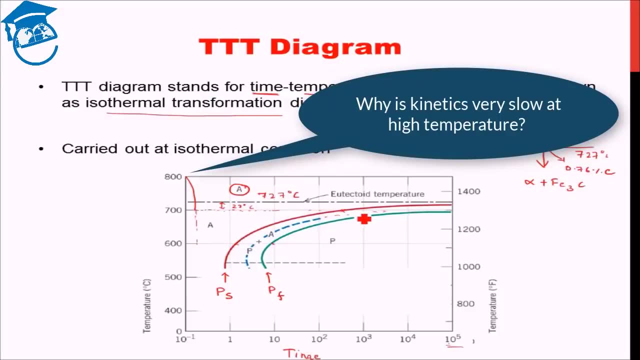 austenite over the course of time, and then you have a certain amount of pearlite formed and remaining austenite over the course of time, and then you have a certain amount of pearlite formed, and there then again you might ask: why is it that the kinetics is so slow at high temperature and why is 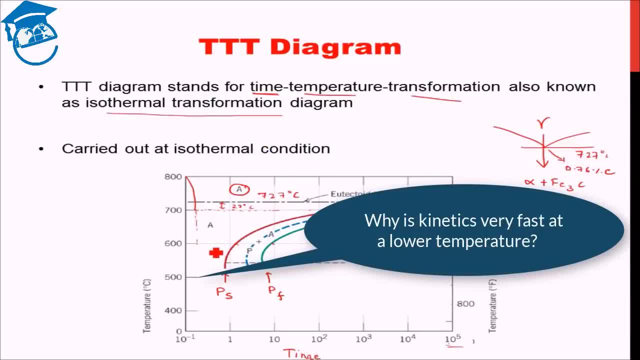 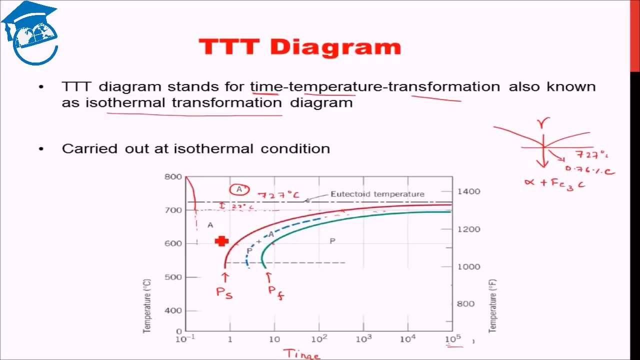 it that the kinetics is so fast at lower temperature? shouldn't it be the opposite? shouldn't it be that at higher temperature you have higher diffusion rate and the kinetics should be high, that is, the pearlite formation should be quicker. okay, so just to give you the idea, there are two. 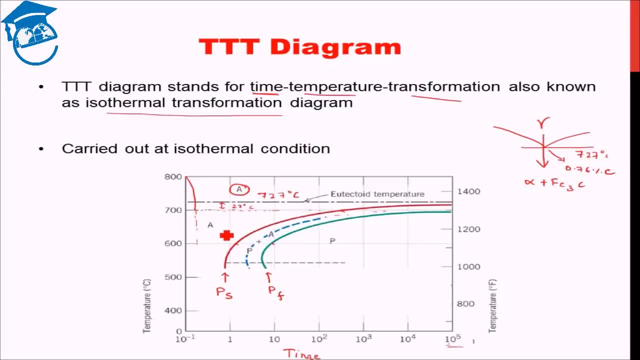 competing processes here. rather, there are two steps involved, as we discussed beforehand. one is nucleation and second is growth. as i said previously, for nucleation you need under cooling, you need to have a driving force under cooling less the under cooling more nucleation will take time to 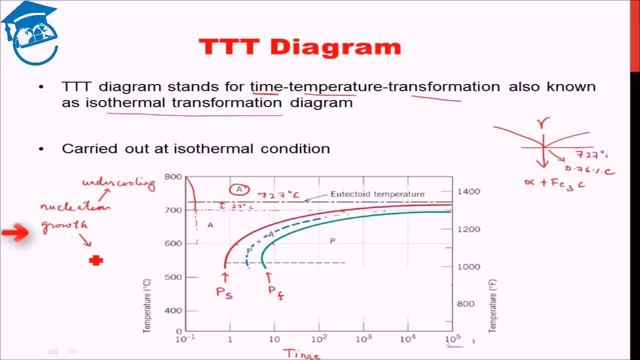 occur. growth is diffusion based. diffusion based, so for growth, higher temperature, faster the process. so what exactly is happening here is that nucleation is kind of the deciding factor in how much time it will take. the nucleation of pearlite is taking a lot of time at higher temperature. 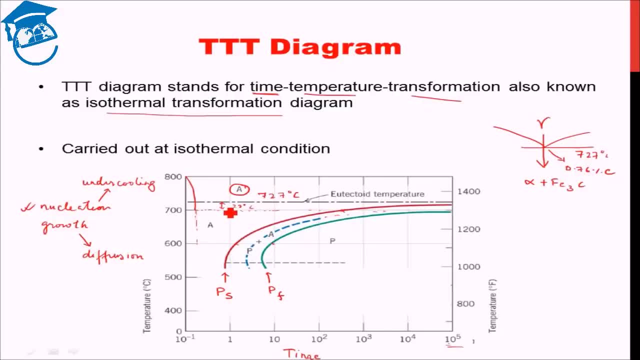 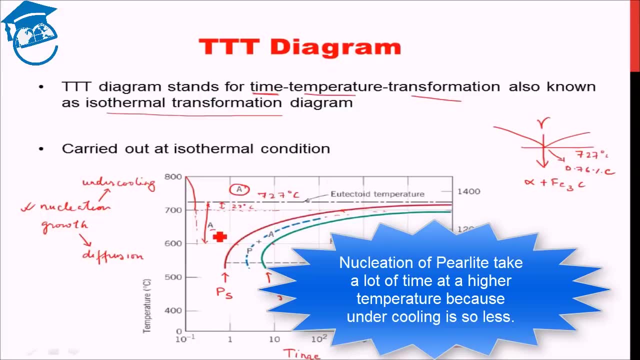 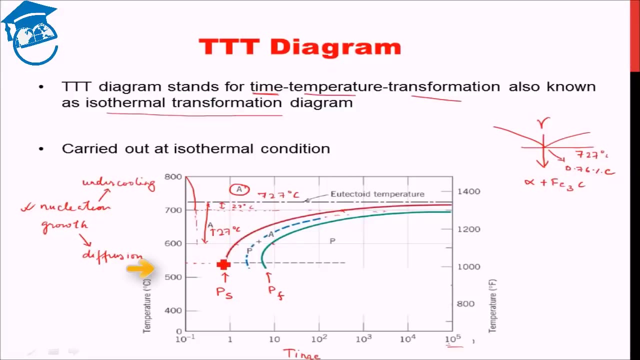 because the under cooling is quite less. at 700 degree celsius we have 27 degrees celsius and 27 degree under cooling, whereas at 600 degree celsius we have 700- 127 degree celsius under cooling. this pearlite formation takes place till around 550 degree celsius. we will see what happens below. 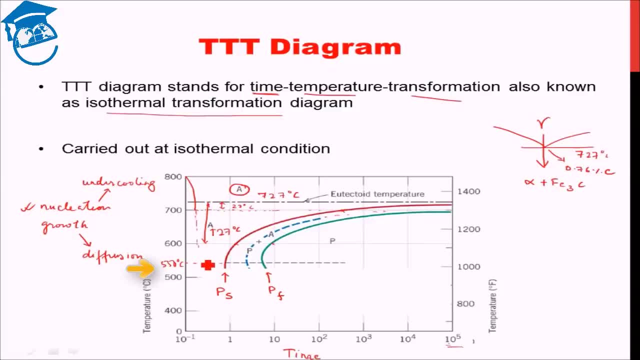 that later. so at 550 degree celsius, we have a under cooling of 177 degree celsius. so what we see is that as we lower the temperature and we lower the temperature, we have a under cooling of 50 degree celsius. at 500 degree celsius, and as we approach 550 degree celsius, the under cooling 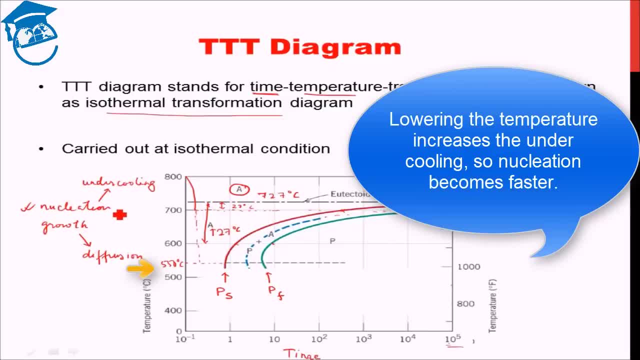 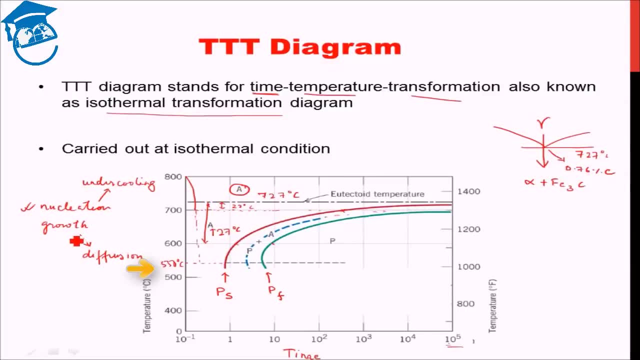 increases. thereby nucleation does not take much time. okay, and though the growth is diffusion focused growths, that it's deciding factor is diffusion. still, 550 degree celsius in itself is a quite high temperature, so the diffusion rate does not vary drastically between 550 Celsius and 700 degree Celsius. so basically, growth does not take a lot of. 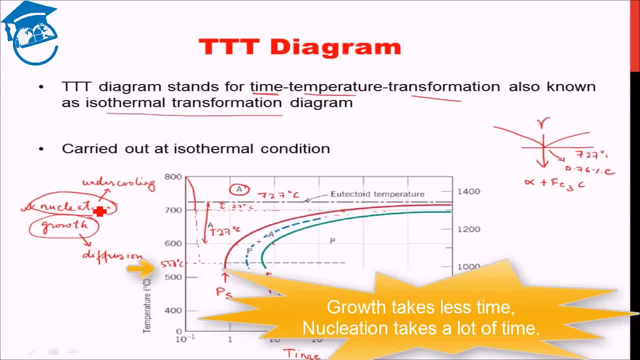 time. nucleation takes most of the time. therefore, higher temperature requires a lot of time to form nucleus. thereby the process of pearlite formation takes a lot and lot of time. lower temperature: nucleation driving force is much more higher. nucleus are formed immediately. diffusion is still quite high rate. 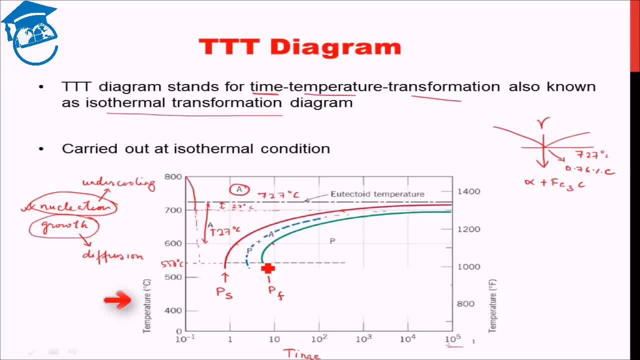 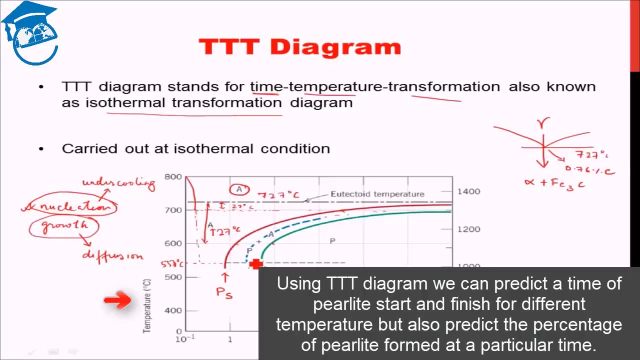 thereby the pearlite formation is quite rapid. fine, so we see that using the TTT diagram, not only can we predict at what time we will have pearlite start, at what time we will have pearlite finish for different temperatures, but also we can predict at any intermediate time what percentage of perlu is formed and what. 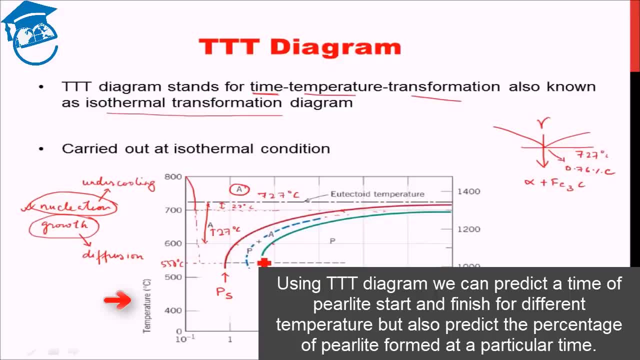 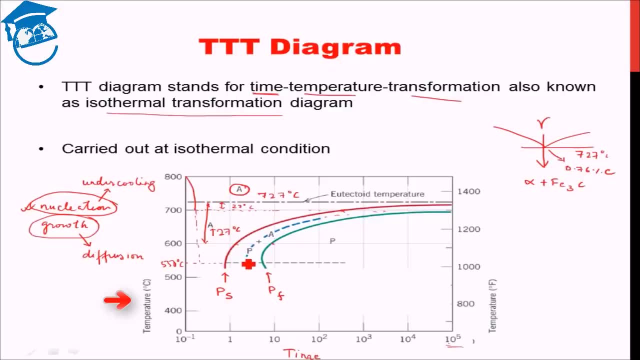 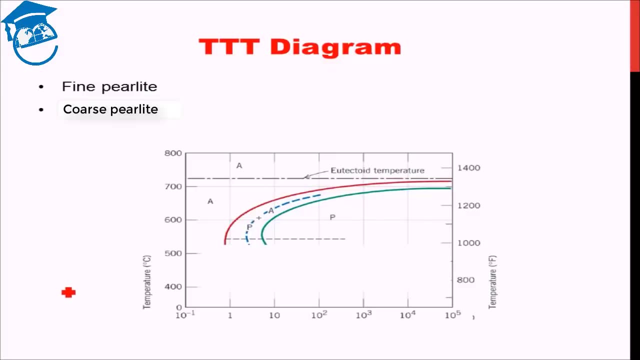 percentage of austenite still remains in the sample, In the same way, when we put the chance, all right, of mon energizedourage system. With this background, let us see something more now. I just discussed that we have pearlite formation up till around 550 degree Celsius. right, But there are actually two types of 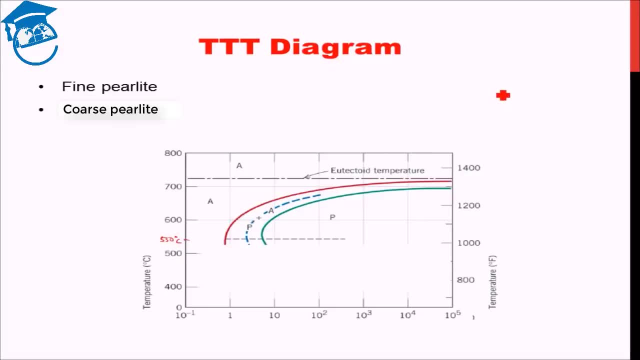 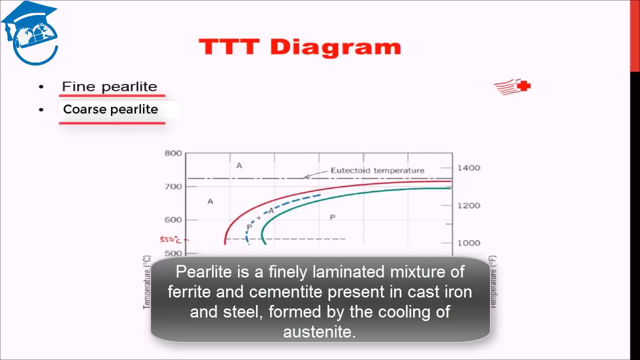 pearlite. If you remember from previous lectures, pearlite is basically a lamellar structure with alternating layers of ferrite and cementite. So you have ferrite and you have cementite. But- and we know that ferrite is to cementite- ratio of width is 7, is to 1. But the cementite 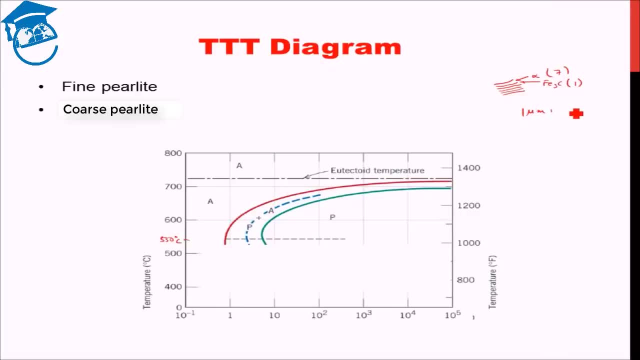 can be 1 micron and ferrite can be 7 micron, or the cementite can be 10 micron and the ferrite can be 70 micron. The ratio needs to be maintained, but we do not know each of them is how thick, So it 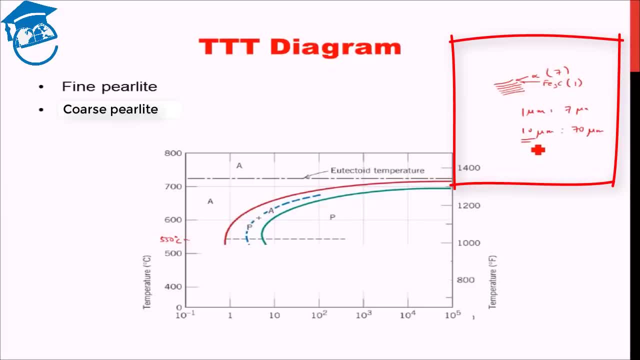 can be really, really fine. It can be quite coarse in structure. How do we find out, or what decides, whether the pearlitic structure will be fine or coarse? That is decided by what temperature we are holding and trying to form the pearlite. It is basically depending. 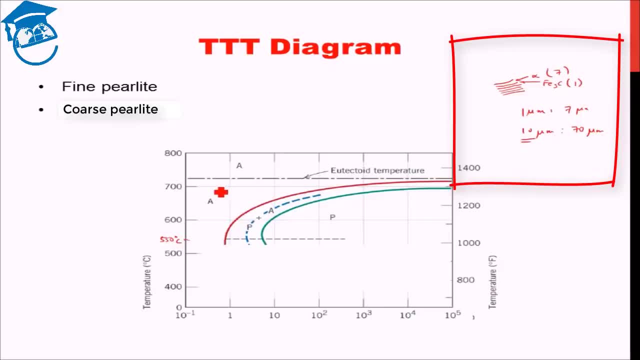 on the isothermal hold temperature Again, as you have to temperature like at 700 degree Celsius. what is happening? we have a lot of very high temperature. thereby diffusion can take place over large range, large distances, right, But the number of nucleus formation is quite slow. Nucleus formation of nucleus. 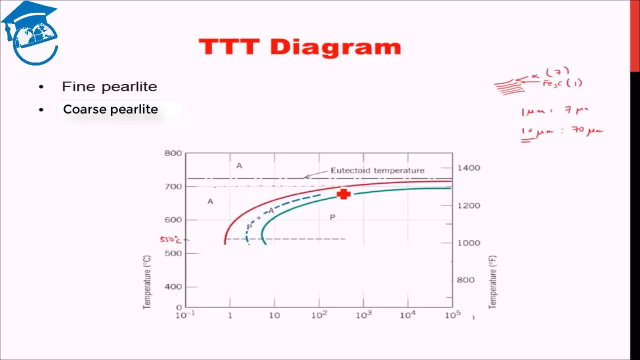 is very less because of no driving force. Thereby the number of nucleus formed will be less by 0.3 instant繼續 gör machines. therefore, number of nucleus is still there. 0.3 instant is correct, But the number of nucleus. 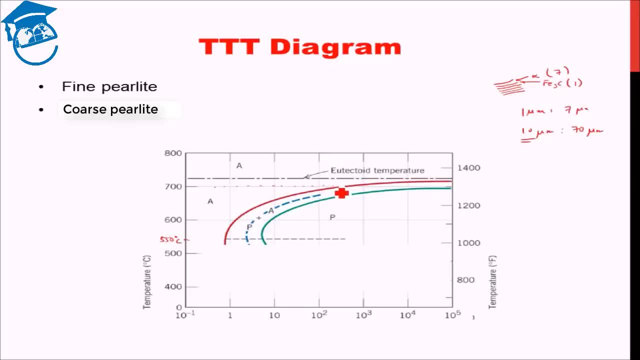 forms won't work out because of low firing force, So we use for thestyroid guys. it is generally 2 degree Celsius tässä. What happens now? the boutique becaese the strand temperature, But the diffusion rate, possibility of diffusion, is more. Therefore, what happens at higher temperature is that we get coarse pearlite. Coarse pearlite Because we have less number of nucleus and the diffusion of carbon from ferrite region to cementite region can be easily done. 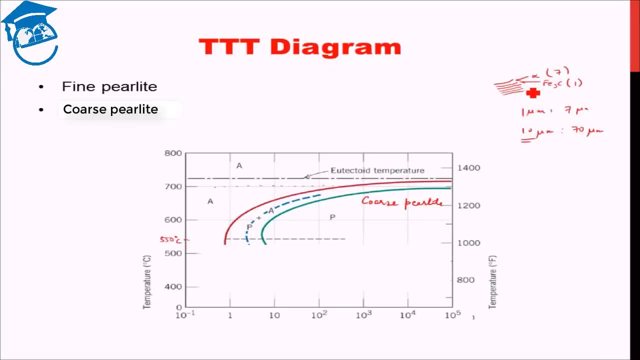 Therefore they can be separated by larger distance. Thereby we have coarse pearlite, But at lower temperature. what we have is that we have a lot of driving force. Many, many nucleus originate Thereby. the nucleus are quite close to each other and that added to the fact that diffusion is slower at lower temperature. we have fine pearlite. at lower temperature. 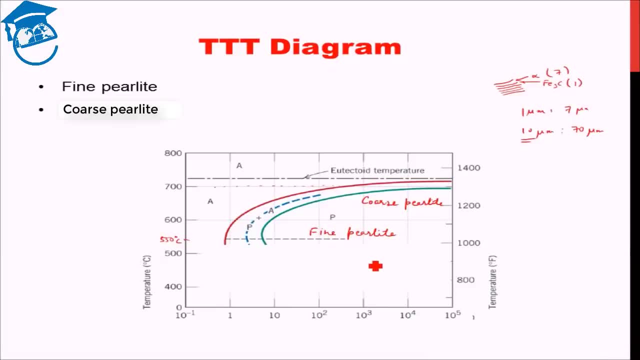 Coarse pearlite. So this gives you an idea where we will have a coarse pearlitic structure and where we will have a fine pearlitic structure. We will not go into the details of exactly how the property varies between coarse and fine pearlite. We will see that briefly later. 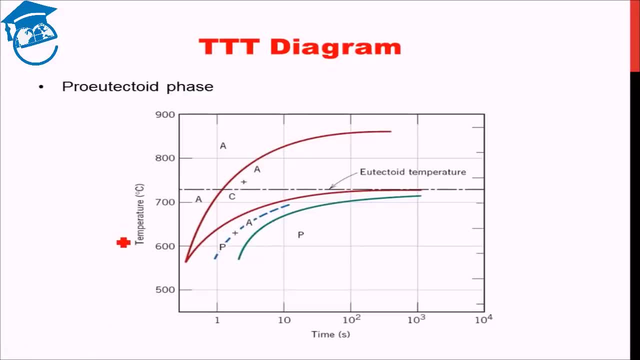 Now the previous two diagrams which we discussed. we were discussing about The eutectoid phase, Eutectoid composition. We were discussing about 0.76%. But what if we are at a different region? What if we are at, let's say, 1.1%? Then what will happen? The thing that will happen at that time is: let me draw that region again. 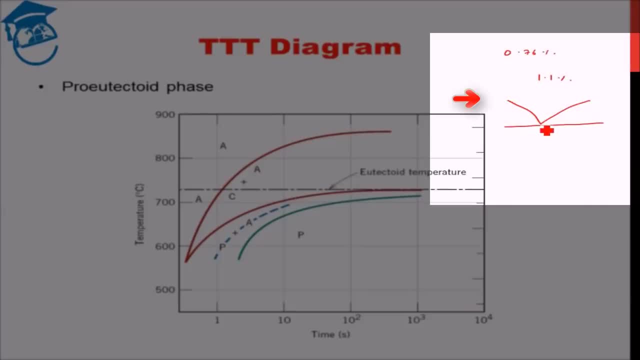 This is 0.76%. So this is 7.1% carbon. This is 7.27 degrees Celsius. Here we have gamma, Here we have gamma plus Fe3C, and let's say we are at 1.1% here. 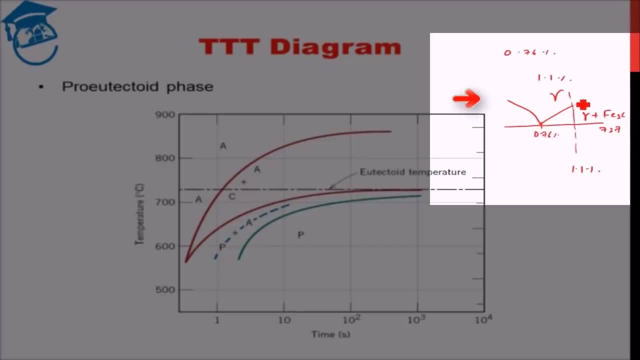 Then initially we have 100% gamma, That is austenite. But in this region we form austenite plus cementite, That is, austenite remains and cementite is formed additionally. This is called as proeutectoid cementite. 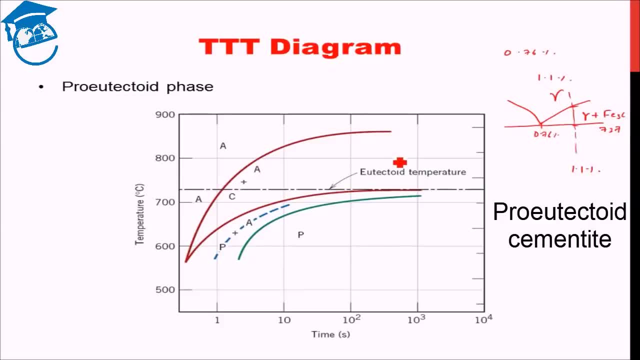 you remember that is reflected in TTT diagram also. what is happening is: you suppose you are isothermally treating it at at this temperature, let's say 750 degrees Celsius, so we basically cool it from, let's say 800 to 750 degrees Celsius and we hold it at that temperature initially till one second. it. 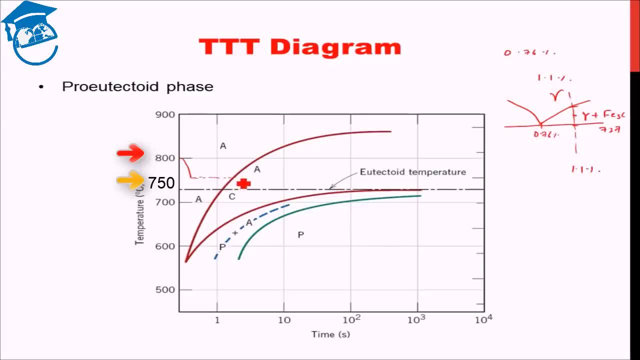 is hundred percent austenite, but at around three to four. second, what we see is that cementite starts to form, that since we are at this region, we should have cementite, but that cementite formation is also a diffusion driven. therefore, there has to be a kinetics which leads to this slow down. and now if 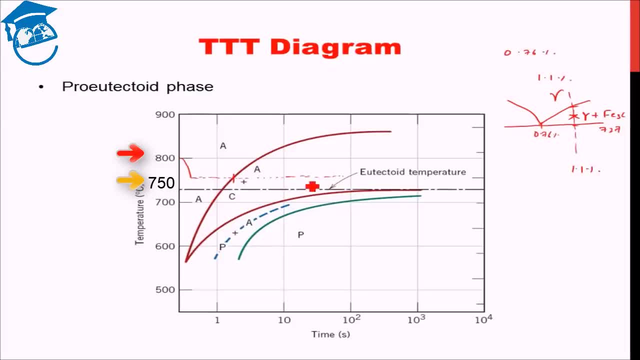 you maintain the temperature, we get the cementite. we form the requisite amount of cementite that should be formed over there. this is the pro eutectoid cementite. so this region we have gamma, that is, austenite plus pro eutectoid cementite. fine, now suppose, instead of: 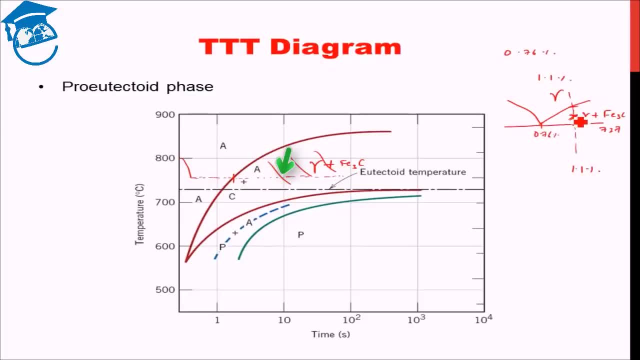 isothermal hold at here. if we isothermally hold it somewhere over here, somewhere over here, what will happen again is that obviously there will be some pro eutectoid and N isothermal isothermal. isothermal is sort of like a eutectoid cementite formation before it hits the pearlitic formation, start curve This. 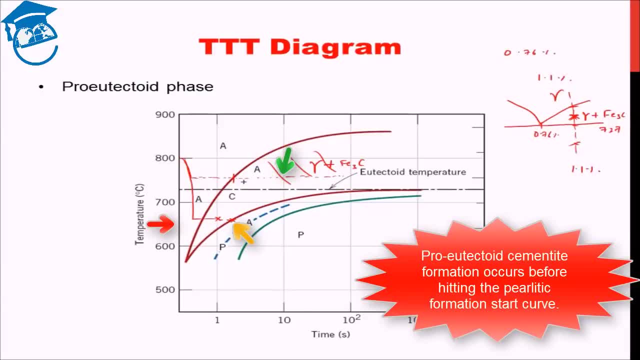 is where the nucleation of pearlite occurs for the first time and pearlite starts to form. Furthermore, it is the same diagram as before. The only difference here was that, due to the hyper eutectoid scenario, we will have the pro eutectoid phases formed. This: 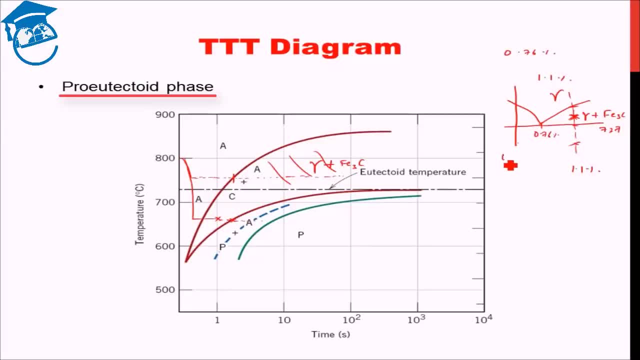 would have been the same if we took a composition over here, let's say 0.5%. Then instead of pro eutectoid cementite we would have pro eutectoid ferrite forming before, But rest of the phenomena would have been on similar lines. 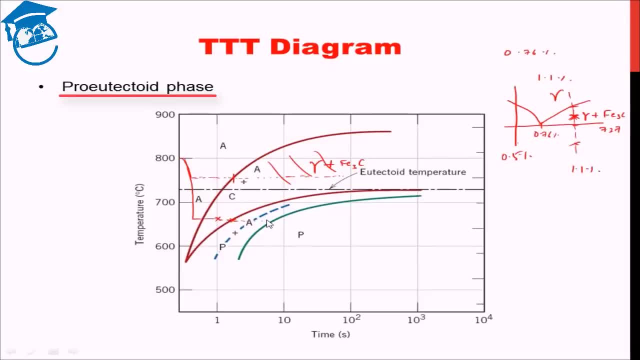 So this gives you an idea about the eutectoid behavior and we saw that in TTT. We saw the pro eutectoid phase formation in TTT also. Now let us see what happens if we go below 550 degree Celsius. I said you that till 550 degree Celsius we have the phase pearlite. 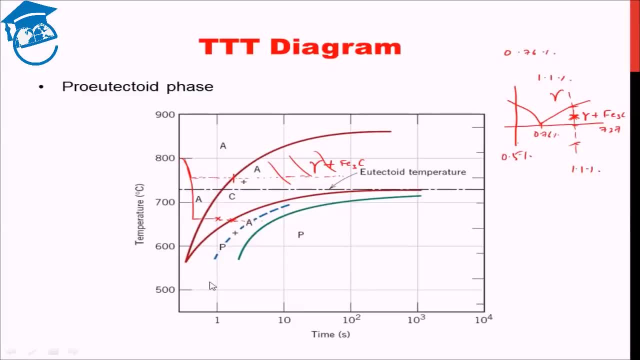 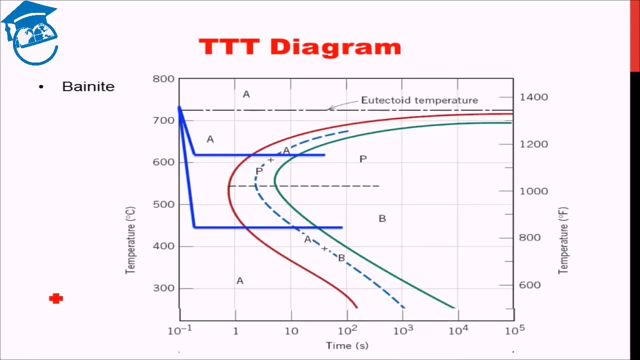 formed, rather the combination of phase pearlite formed. But if we go below 550 degree Celsius, then we have a different kind of phase form. that is known as bainite. If you remember the phase diagram, there was no bainite in the phase diagram. This means that bainite 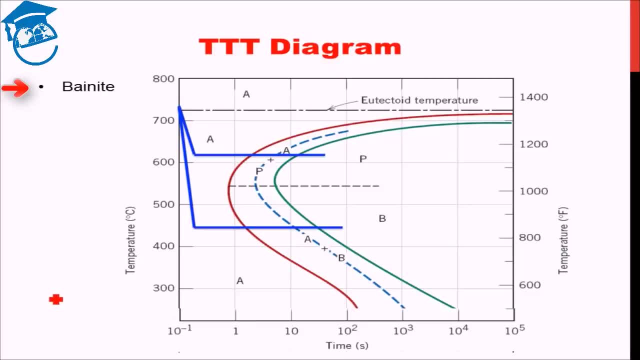 is not the most stable phase. rather it is a metastable phase, But being metastable, it has needle like structure. We will not go into the details of that. It has a much higher strength and hardness than pearlite And thereby using this heat treatment when we require. 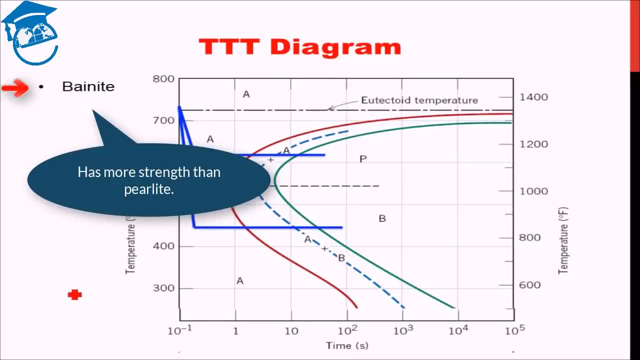 higher strength, higher hardness than pearlite. we actually form bainite rather than pearlite. We do not isothermally cool at it, cool the austenite above 500 degree Celsius. Rather, we cool it below 550 degree Celsius. What we do is this: just to show you, this is the 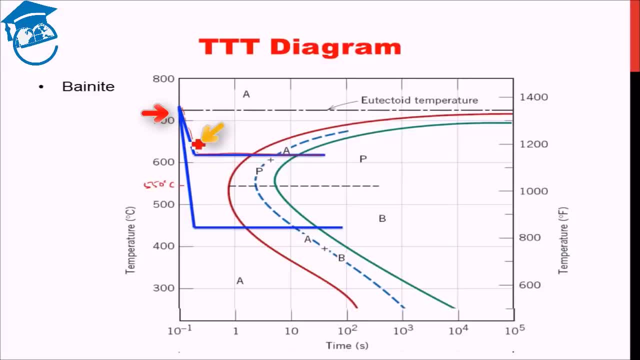 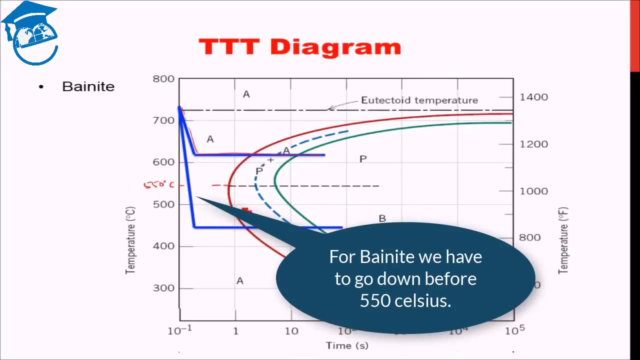 formation. isothermal curve for benite you go below 550 degree Celsius. 550 degree Celsius is kind of a nose. beyond that the kinetics slows down again. why till here? till 550 degree Celsius? the kinetics was governed by the amount of time taken for nucleation. below this temperature, the kinetics is governed by 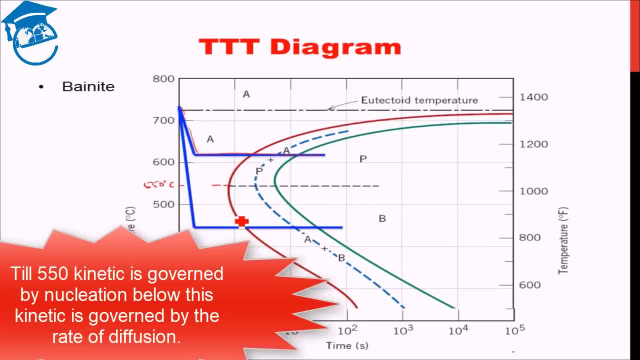 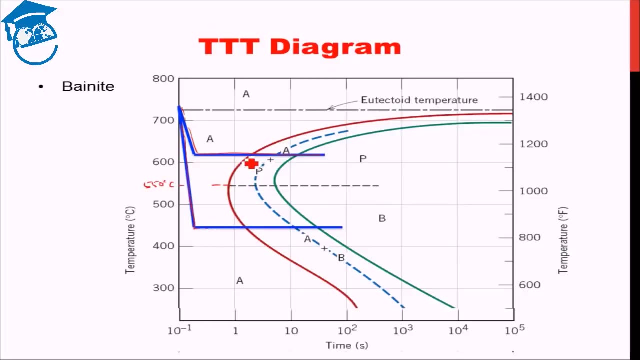 rate of diffusion. if you remember, I discussed about nucleation and growth. so this was driven by nucleation, this is driven by growth kinetics. so what we do is we come at a lower temperature and we cool, similar to pearlite start and pearlite finish. we have benite start and benite finish, we cool it. let's say we are at 450. 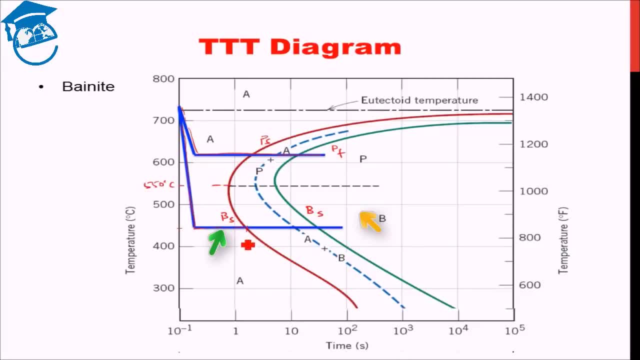 degree Celsius. at around 2 seconds, we start from forming benite. till that time we had 100% austenite. at around, let's say, 10 days, 10 seconds, we have 50% benite formation. at around 50 second, we have 100% benite formation. ok, so we see that the driving force is. 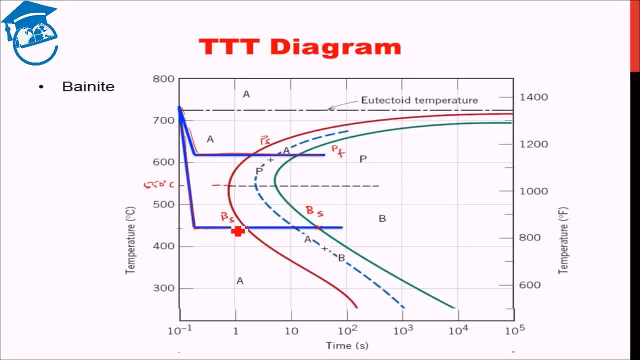 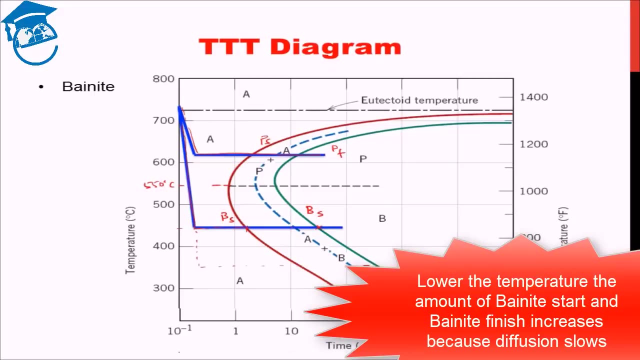 sufficient for nucleation. now, whatever is driving is the rate. what is driving the kinetics is the rate of diffusion. so as we further lower the temperature, the amount of time required for benite start and benite finish keeps on increasing, because now that diffusion is really really getting slowed down, further down temperature, further more. 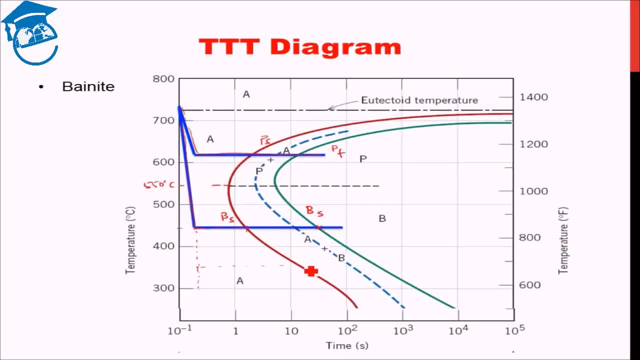 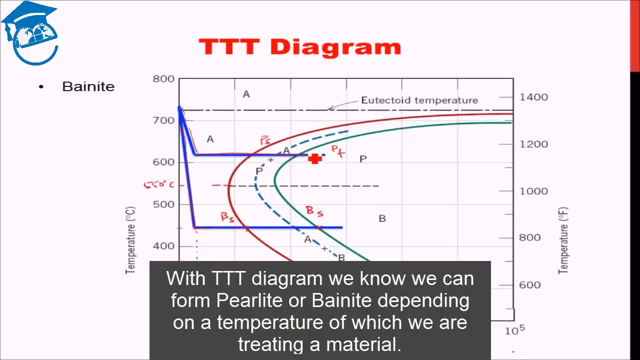 time is required, ok, so with this TTT diagram we see that we can form either pearlite or we can form benite, depending on what temperature we are treating the material. So this TTT diagram is very, very handy to understand the different heat treatment processes. 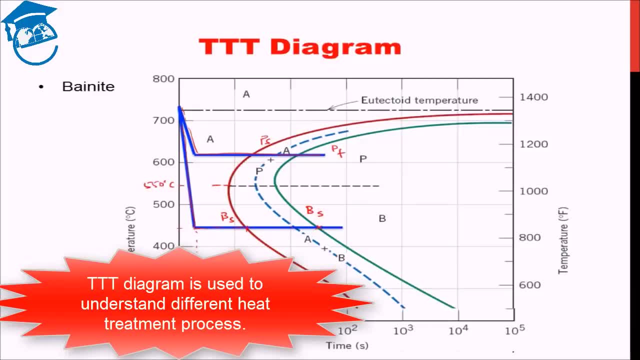 We will also see a different kind of phase altogether. Today we discussed about pearlite and bainite. We will see something which is known as martensite, which is not formed by diffusional processes. Martensite is a diffusion-less process. formation of martensite. 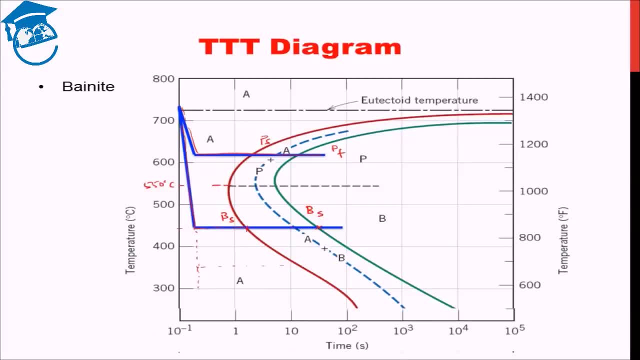 Therefore, martensite formation is actually supported at quite low temperatures. We will see that in a later lecture. Hopefully you understood the concept of TTT diagrams and why we need TTT diagrams. With this background we will continue our next lecture. 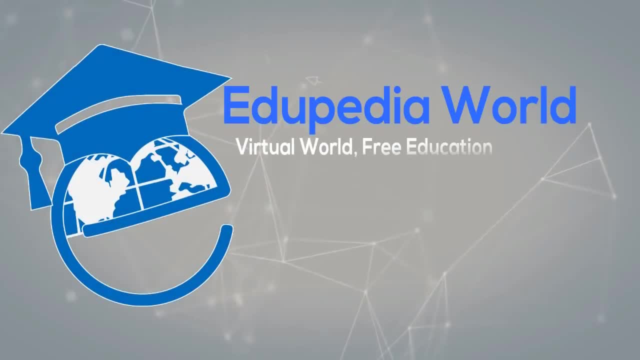 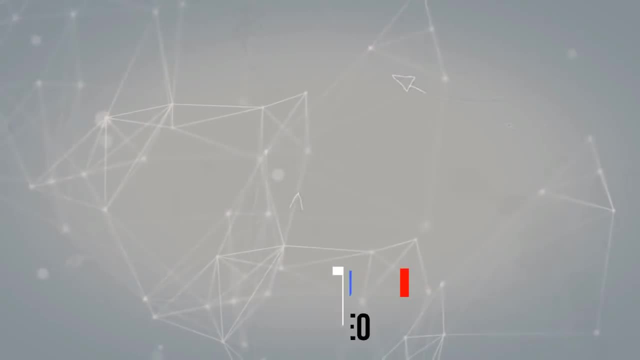 Till then, have a great day, Goodbye. Transcription by CastingWords.